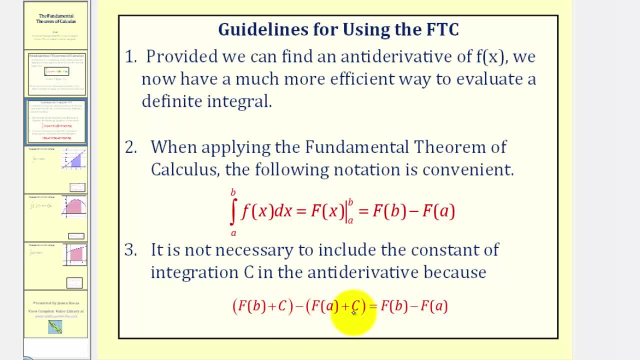 when we find this difference, the constant would simplify to zero, leaving us with big F of b minus big F of a. Let's look at some examples. We want to evaluate the definite integral and notice how the integrand function graphed here on the right. 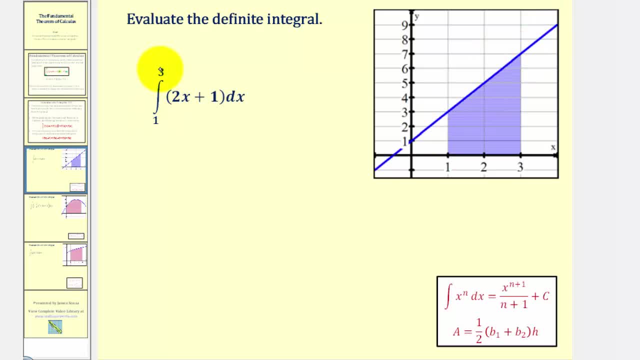 is non-negative on the closed interval from one to three and therefore this definite integral is equal to the area below the function bounded by the x-axis over this closed interval. And notice how this region is a trapezoid, so we could evaluate this using the area formula for a trapezoid. 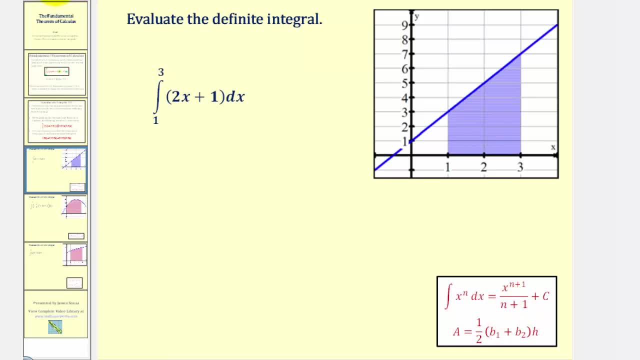 but let's use the Fundamental Theorem of Calculus first. So to apply the Fundamental Theorem of Calculus, we first want to find the antiderivative of two x plus one with respect to x, So we'd have two times. this is x to the first, so we'd have x to the second. 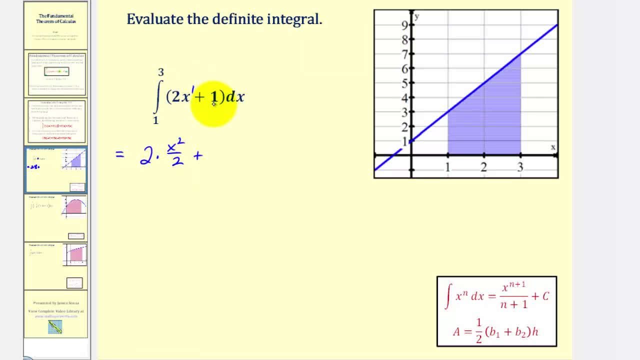 divided by two plus the antiderivative of one with respect to x would be x. We now need to evaluate the antiderivative at three and then subtract the value of the antiderivative at one. But before we do this, let's go ahead and simplify here. 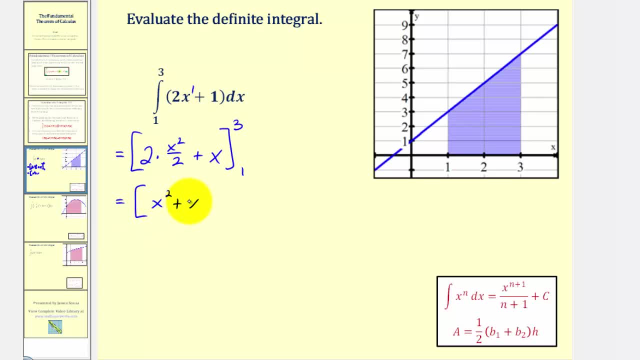 This simplifies to just x squared plus x. So now we'll evaluate the antiderivative first at three, then at one, and then find the difference. So when x is three, we'd have three squared plus three. When x is one, we'd have one squared plus one. 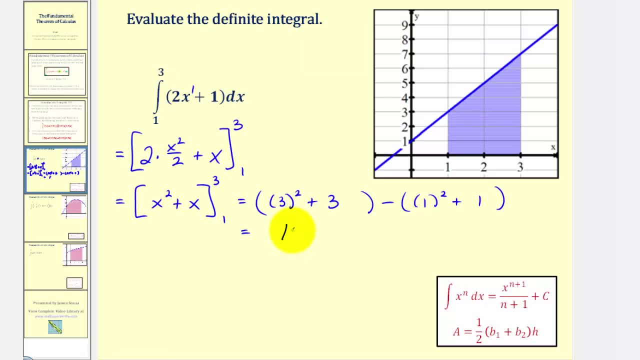 Simplifying: here we have three squared plus three, that's twelve, minus. here we have one squared plus one, that's two. So the value of the def integral, which is also this area, would be ten. Now for this first example. let's verify these results. 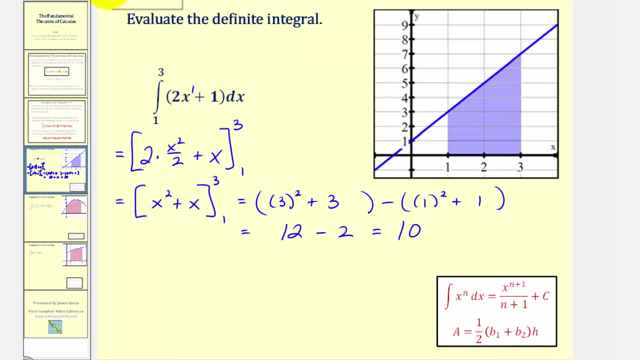 using the area formula for a trapezoid given here. So let's call this b sub one, b sub two, and this would be the height of the trapezoid. So using our formula we have the area is equal to one half. 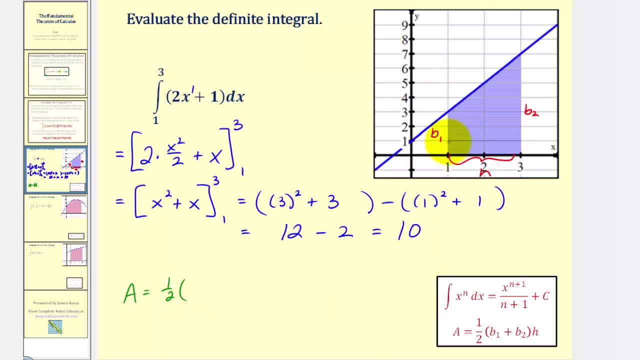 times the quantity b sub one plus b sub two, that would be three plus seven, and the height is two. So we have one half times ten times two, which is ten, Verifying our answer is correct. Let's take a look at another example. 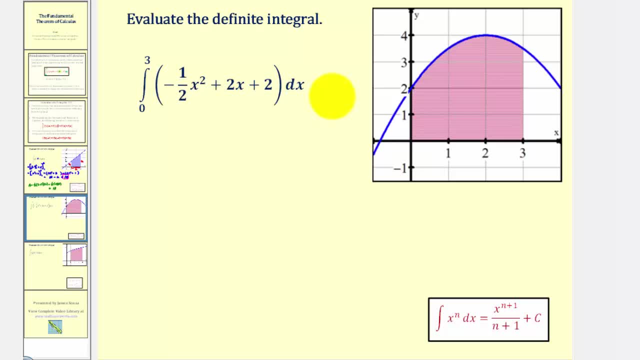 Again, notice how the integrated function is non-negative over the closed interval from zero to three. So this def integral is equal to this area here. So, applying the fundamental theorem of calculus, we'll first find the antiderivative of negative one half x squared plus two x plus two. 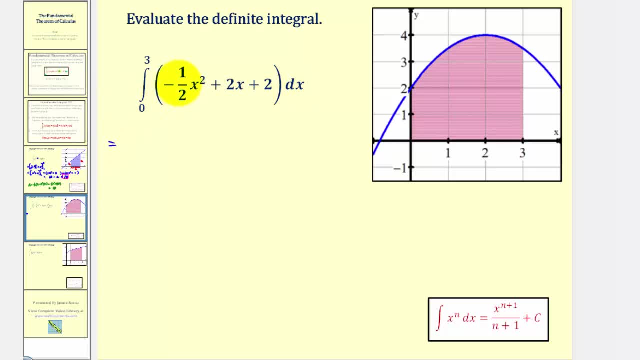 with respect to x. So we have negative one half times x to the third, divided by three plus two times this is x to the first. so we'd have x to the second divided by two plus the antiderivative of two with respect to x would be two x. 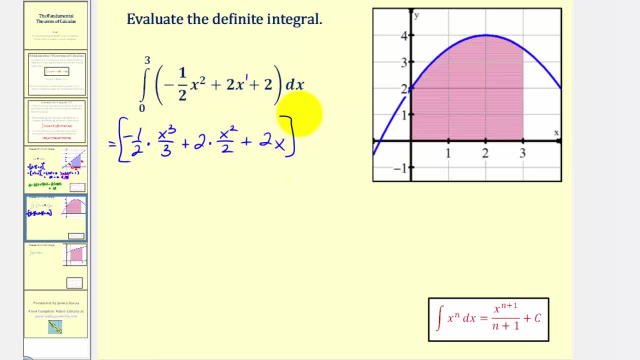 So this is our antiderivative, which we now need to evaluate at three, then zero, then find the difference. but of course we'll simplify this first. So here we have negative one sixth x to the third plus. this would be x squared plus two x. 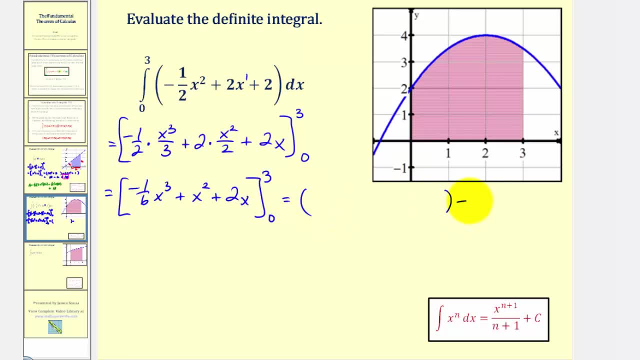 So again, we'll evaluate this at three and then subtract the value at zero. So when x is three, we have negative one sixth times three to the third, plus three squared plus two times three. And when x is zero, notice how each term would be zero. 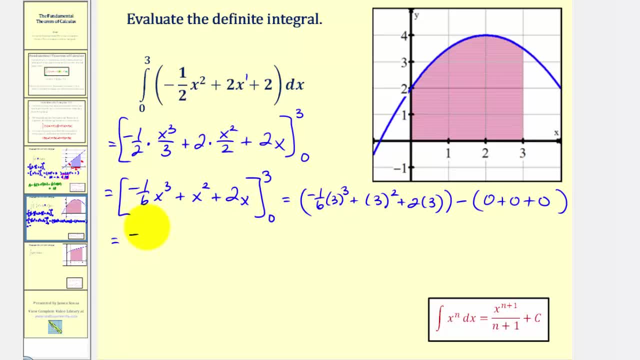 So simplifying we have. this would be negative. one sixth times twenty-seven, which would write us twenty-seven over one, And then we have plus nine and then plus six. Notice how we have a common factor of three here there's. 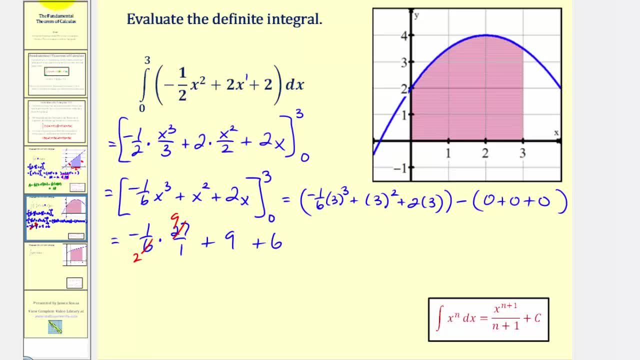 two threes in six and nine threes in twenty-seven. So here we have negative nine halves. this would be plus fifteen or plus fifteen over one. Common denominator is two, so we'll multiply fifteen over one by two over two. 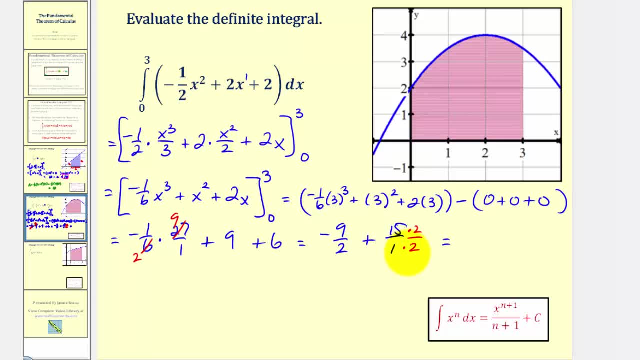 So we have negative nine halves plus thirty halves, which is twenty-one halves. So this is the value of the def integral and because the integrand function is non-negative on the closed interval from zero to three, the area of the shaded region is twenty-one halves. 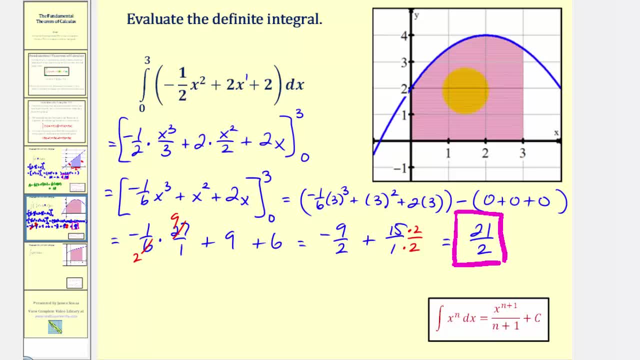 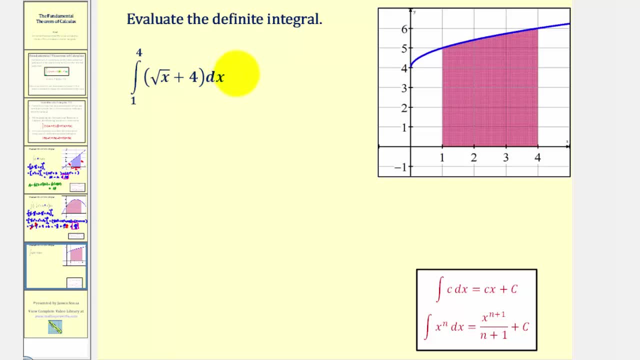 square units or ten and a half square units. Let's take a look at one more example. We want to find the def integral of the square root of x plus four, integrated with respect to x from one to four. Once again, notice how the integrand function is. 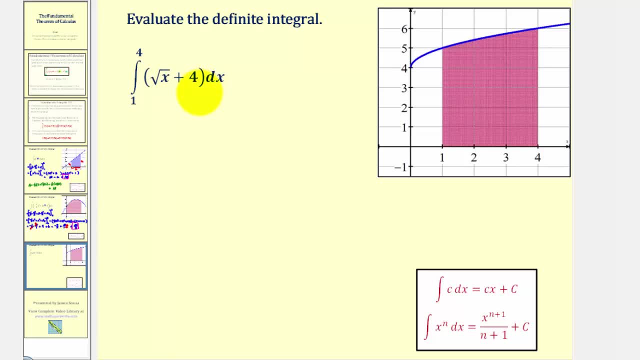 non-negative on this closed interval, so the def integral is equal to this area here. Before we find the anti-derivative, though, we want to write the square root of x using rational exponents. where the exponent of x is one, the index is two. 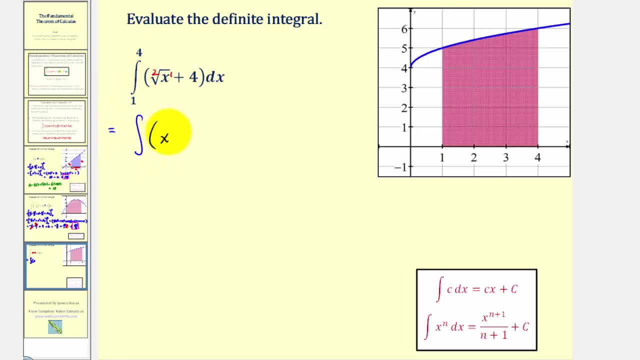 So we can write this as the integral of x to the one half plus four, integrated with respect to x from one to four, And now we'll find the anti-derivative function with respect to x. so for x to the one half we'd have x to the power of one half plus one. 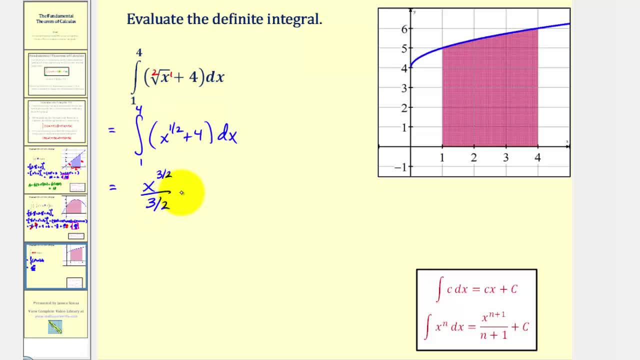 that's three halves divided by three halves plus the anti-derivative of four is four x. But dividing by three halves is equivalent to multiplying by two-thirds, so we'll write this as two-thirds x to the three halves plus four x. 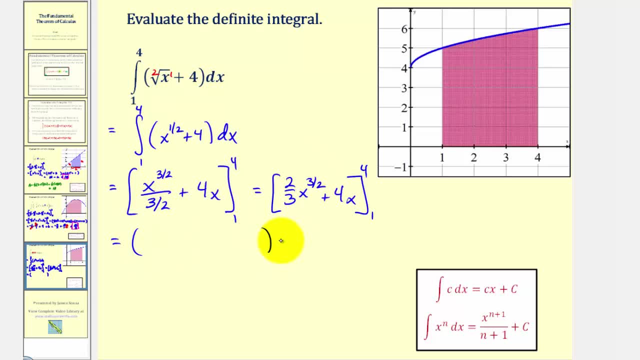 And now we need to evaluate this first at four and then subtract the value at: x equals one. So when x is four, we have two-thirds times four, to the three halves plus four times four. And then when x is one, we have two-thirds. 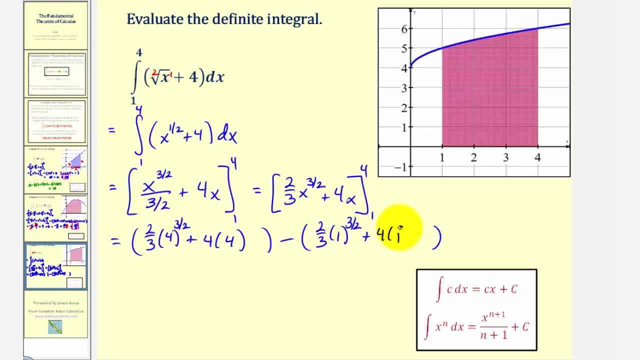 times one to the three halves, plus four times one For four to the three halves. that's equivalent to the square root of four to the third, which would be two to the third or eight. So here we have two-thirds times eight, that would be sixteen-thirds.